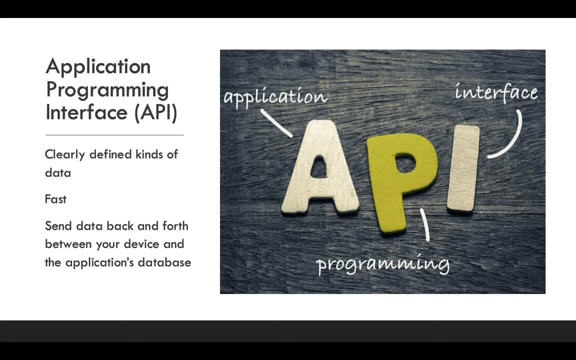 Web APIs provide a mean of communication between websites and users structured by some rules. Web APIs provide a mean of communication between websites and users structured by some rules. In particular, they allow users to obtain clearly defined kinds of data quickly and by requesting. 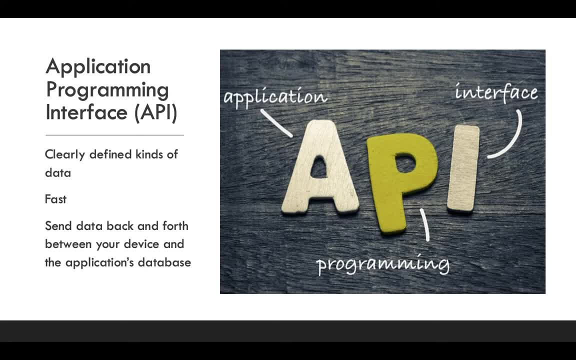 it directly from the database underlying a particular website, And keep in mind that it is not necessarily because the companies are very kind at allowing you to do this. At the same time, there is an interplay between the customers and the website. Basically, you're receiving the data. 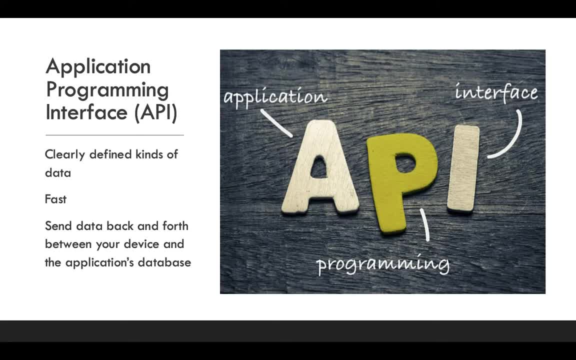 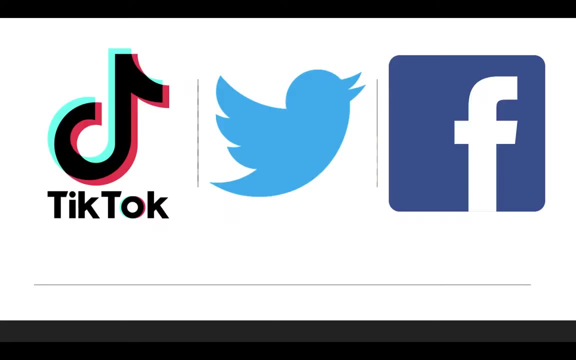 from them. You're also sending some data to their database. So in this video we are mainly focusing on the APIs that deliver data from the website to users, And many major companies have already started giving APIs to the customers, especially the developers they want. who wants to get some data from their 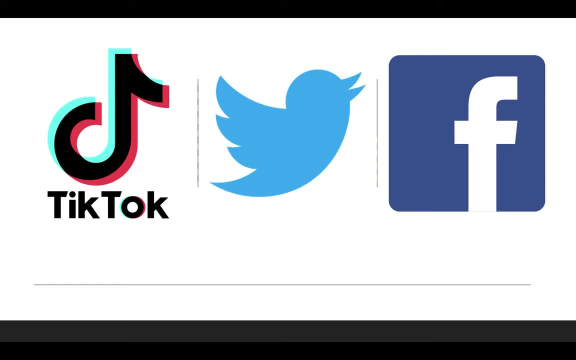 platform and do some meaningful analysis on them or build an application that is useful. TikTok, Twitter, Facebook are also some examples. I mean to get the API you need to go through an application form or some process for them, but still it is manageable at the end to get access to their data. 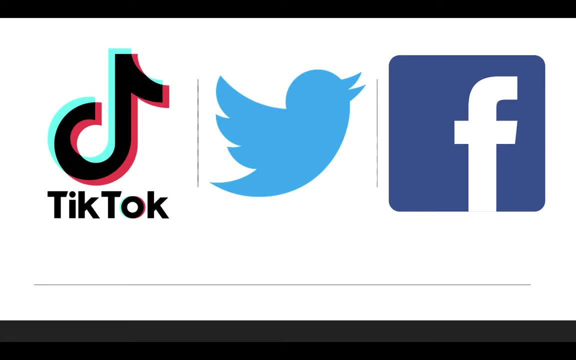 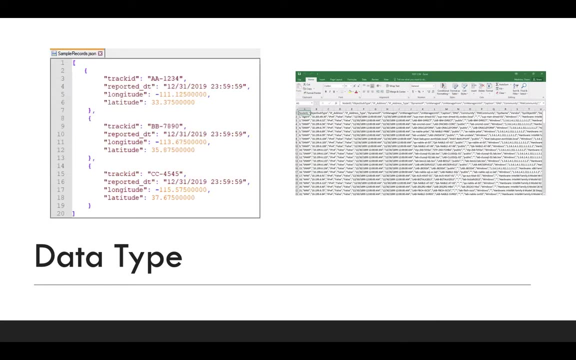 And these companies, alongside many governmental agencies, have created public APIs Which provide easy access to their data SPEAKER 1 to encourage developer to use their platform. so apis provide data in various formats. for example, json probably is the most popular format and the reason is that it is useful for structuring the 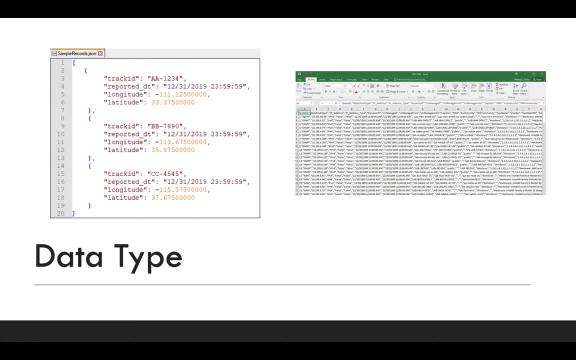 data, because it preserved the hierarchical structure and meta information about the dataset than, uh, let's say, tab or comma separated for files such as csv, i mean, and csv's could be useful. you don't need always the hierarchical data, for example, if you are going to use twitter. 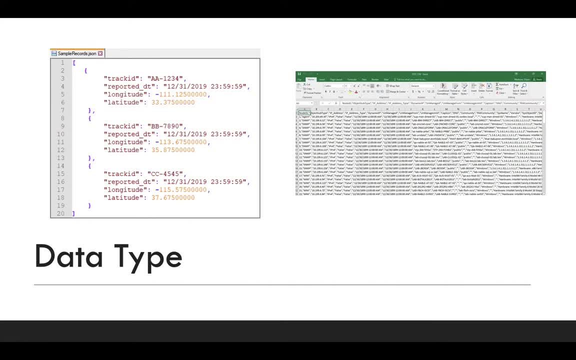 api and get some specific information about certain hashtags, then you don't need all these hierarchies. basically, what you're interested in is that: who used this hashtag, when they used this hashtag, who are they using and what they're using? which one they're using? which one they're using? 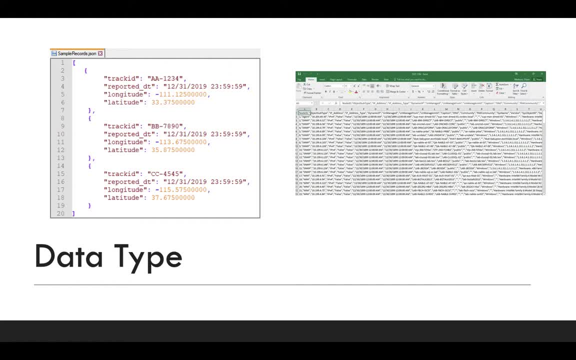 which one they're using, who used this hashtag, when they used this hashtag? when they used this hashtag are their friends. so so these kind of things and it could be very well contained in a CSV file, so it depends really on your use, but JSON is one of. 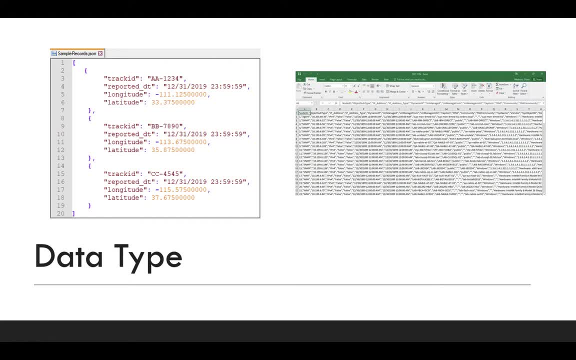 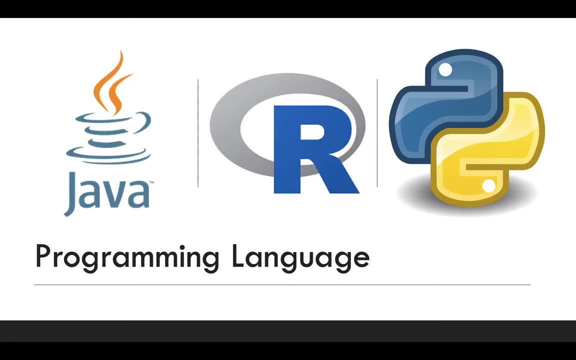 the most popular one, and it also depends on the programming language you're using. for example, there there are libraries that make JSON data manipulation quite intuitive, depending on the programming language that you're using, and talking about the programming language in order to interact with an API efficiently. 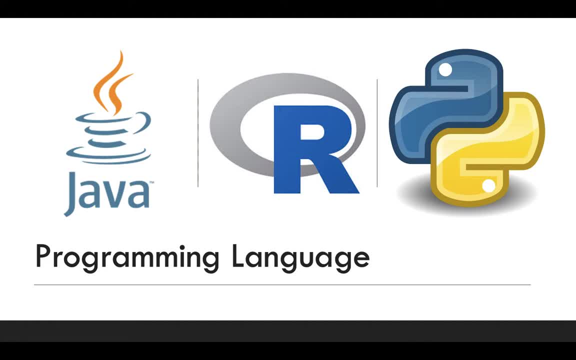 across a variety of computer programs written in different languages, for example Java or Python. researchers rely on API wrappers and these tools which exist for most popular API is a lower researcher- programmer- scientists- to request data directly from an API while using their own programming language of choice. so it helps you not to limit the choice of 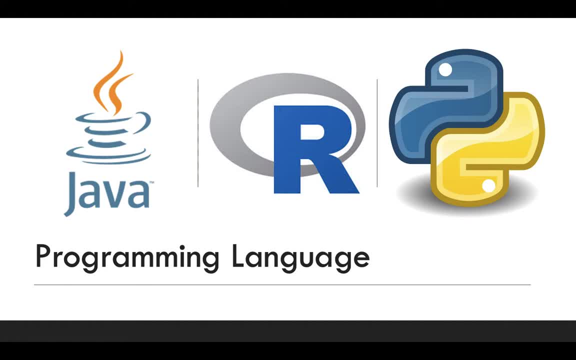 programming languages and you continue working with whatever you have been working up to now. so, as you see, API are somehow another way of getting the data from websites and instead of a web scraping that you saw in the other videos in this lecture and it is. it's quite a straightforward of doing it and 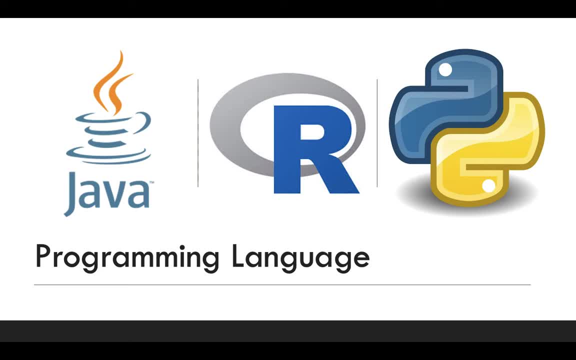 it is pretty simple. there are several examples. for example, Twitter, as I said, is a very popular one, and there's also- there's already- packages. for example, tweet pie is a good tool, a good library, basically in Python, that you could use for getting the data from Twitter. I'm getting back to that at the end of this. 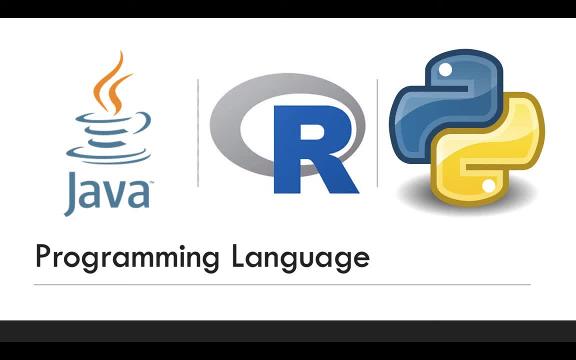 video like how to go there and what to do and where we are standing now. so I'll get back to that at the end of this video like how to go there and what to do on where we are standing now. yeah, but similar to many thing else, api's have also their own drawbacks, not 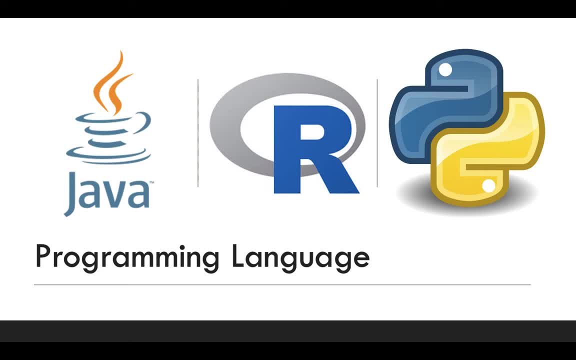 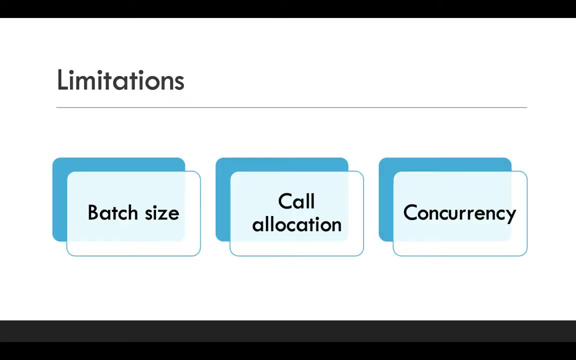 in drawbacks, in the sense that they are not doing what they are supposed to do, but using API come with some sort of limitations and, in short, the limitations are the batch sizes, the call allocation and the concurrency. so what these mean. when you're talking about batch sizes, what we need to consider: the size of the batches which 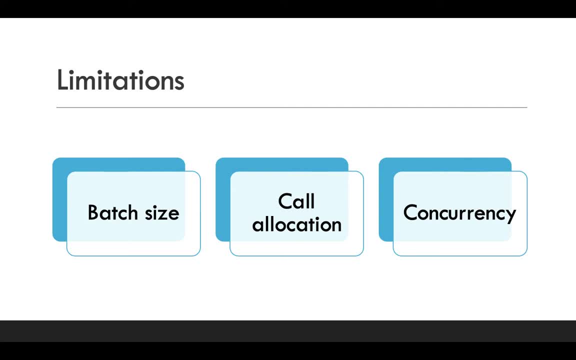 is basically the number of records being requested from the source and being sent to the target application. specific map connectors already have a property to count for these limits, so this is something that you need to be careful. when you're sending your request, you need to be aware what is your. 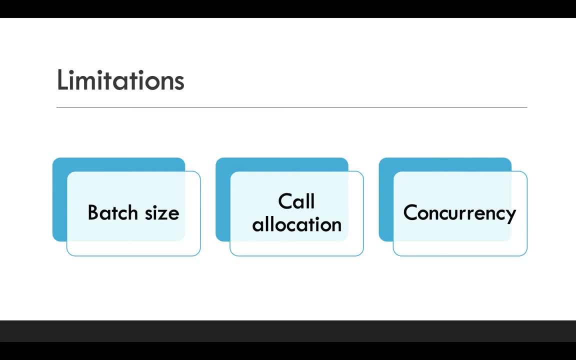 limitations on each request, how many, how many records you could really apply for to get downloaded. basically, what it means is that what whenever you're using an API, you need a bit of planning beforehand: how much data you need to have, how many requests. considering the batch size limit, you could get your data and these sort of things. so it needs a 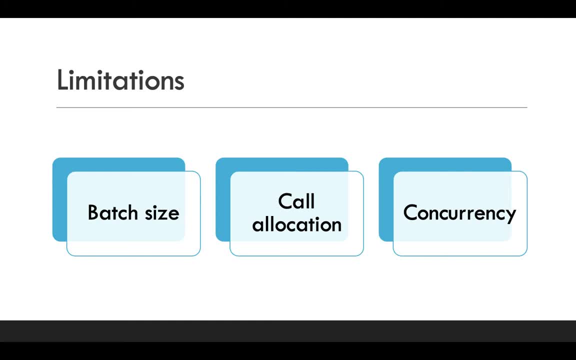 bit of planning before starting to use the API. the other limitation is the call allocation and basically some API is limit the number of calls a user is allotted during a 24 hour period. this means basically that there in the previous limitation, we talked about batch sizes and we said that you 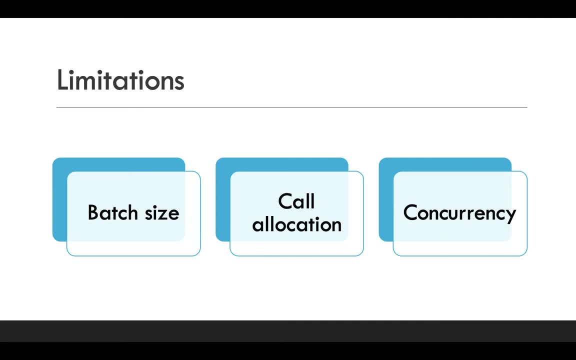 probably could increase the number of your requests that you're sending to data specific website using the API API, so that you could download all the data that you need. but the call allocation could be another problem. I mean, for example, you could decide I'm going to send 100 requests to this. 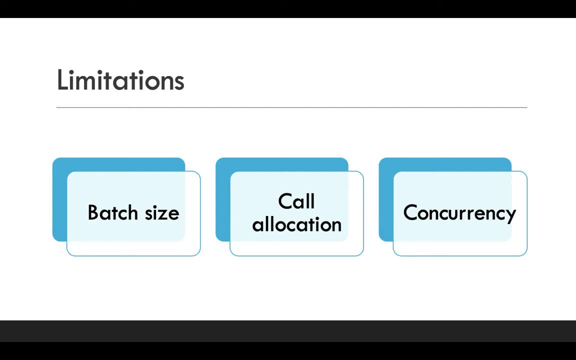 website in these 24 hours and I get whatever I want to get, But there could be a limitation: that 100 is not really actually the number that you could do your call allocation. It could be like, I don't know, 30,, 50,, 20.. So this is another factor that you need to keep in mind when you 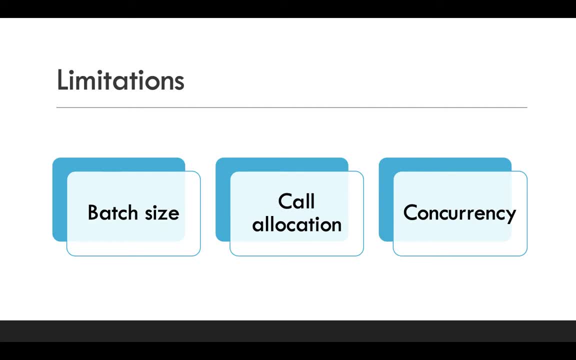 are planning to use APIs. So until now, you need to know two things: What is the limit? number of requests that you could send, number of records that you could ask for and how many times you could ask- basically to get that many records in a day, And that has impact on how you're defining. 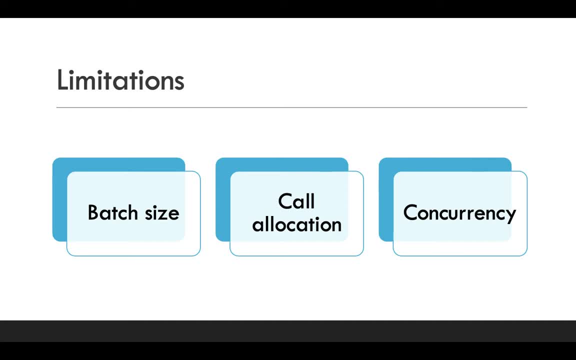 your project. It is basically in this data collection phase, how much time it takes until you could collect all the data that you need to have, And always also keep in mind that things could not go according to your plan potentially, So always have a bit of room to wiggle. 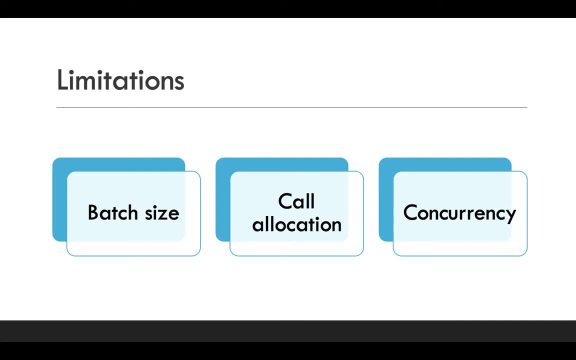 And the last limitation is the concurrency And the APIs may have a limit on the number of active sessions an organization and user can have at any given time. This adds an implied constraint on how you interact with the API during the session, for example. 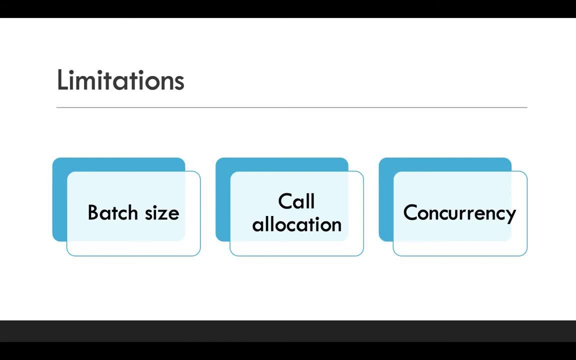 So it depends on if the server is using the same API, conferences and whatever, and depending on the specificполices, I might have that, since you can't see the wrong anymore, But this could also take into account how often the setup error may occur while performing a lookup to. 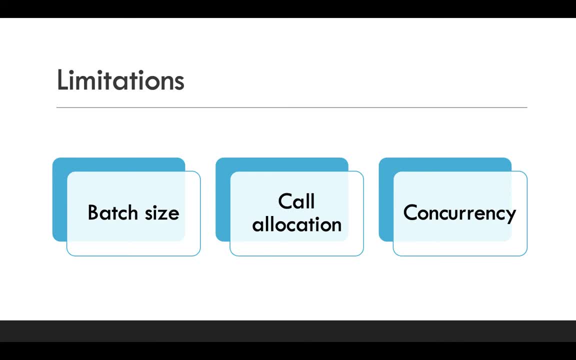 the same API you're using for the source data. So, all in all all these limitations that I said here is about how fast you could get the data It melts down. It would be an ideal life if, basically, there was no limit on the batch size, No limit on the call. 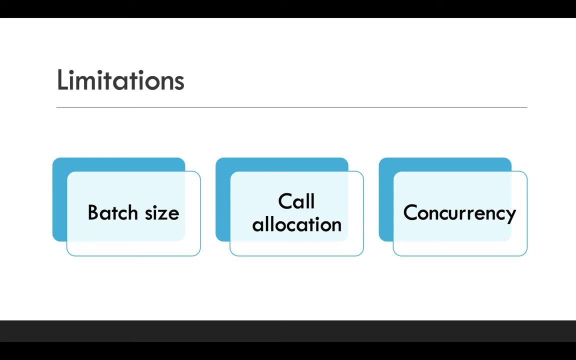 allocation, No limit on the concurrency, Then several users at the same time would send the user the actual data that they receive with the package and anotherís data, that is one day later, will actually get all of the data back, And this situations can also take up certain events. Absolutely. 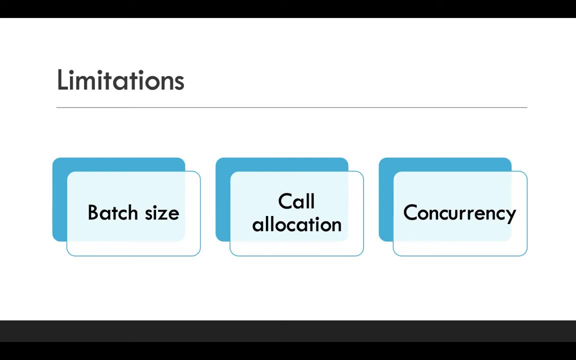 If the error may occur, would send unlimited number of records, or I mean the many that you need, and then they would get it fast. but this is not the reality. you should plan how many people in your team can do it within your organization, how many times you. 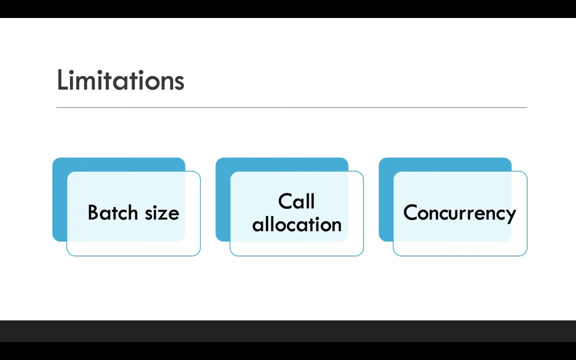 can ask, send requests within a day, and in each request, how many records you could ask for, and all these have impact on how you're going to do that. still, api's are pretty useful when it comes from getting the data from the web, and by that, this is the end of my presentation on using api's. 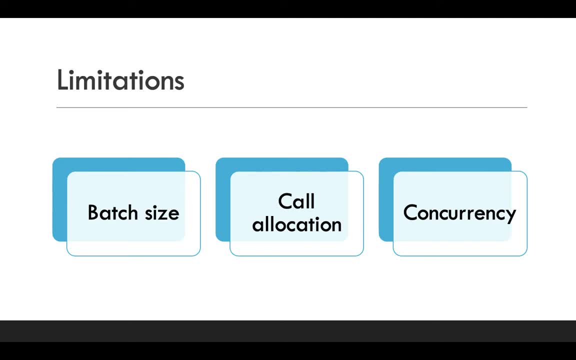 for collecting the data. what I wanted to add here is that we in this lecture, we talked about web scraping, we talked about API, we talked about different tools that we can use to collect data and we talked about some of the things that you're using. you could use for web scraping, but 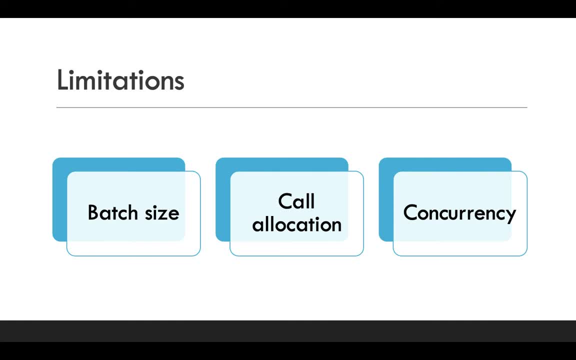 I mean, there are some ready-made solutions, some plugins that you could, for example, install on your Google Chrome and get the data, and, and they are useful. no one says that you need to be very- I don't know uh nerdy tech savvy to be able to get the data you want. so you sometimes could just. 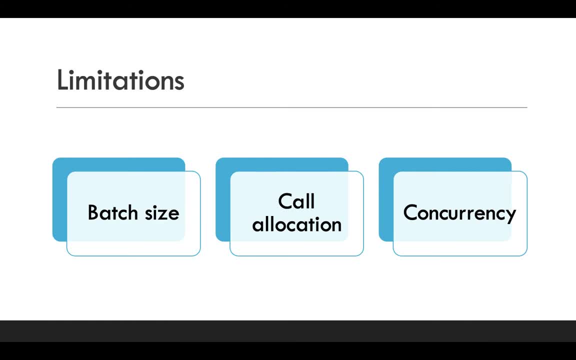 install these plugins and get what you need depends on what you're doing and what you're using and what you're using in your data. so I'm going to talk a little bit about what is it that you are doing as a personal suggestion, if you are doing a, 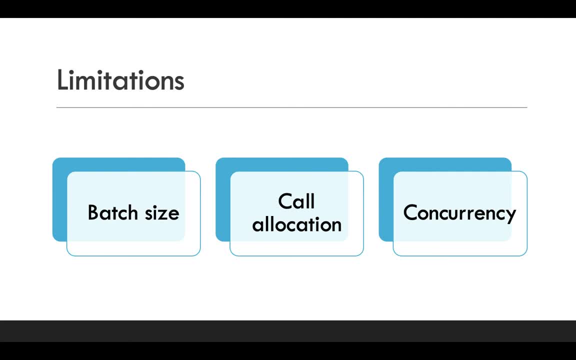 professional project or even a course project, then the requirement is really for you to do the actual web scraping. you're collecting the data through API. don't go for these plugins. but if it is for a personal project and it really doesn't matter how you get the data- it is the data that only matters. 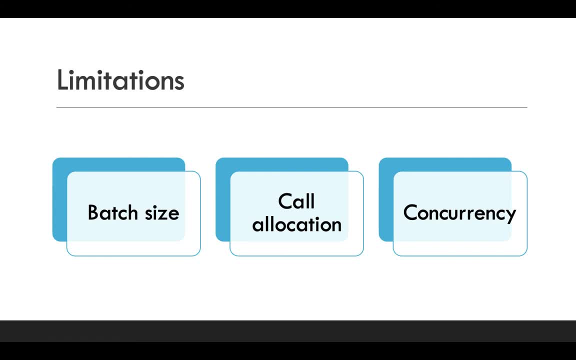 to do to you. you could use these plugins, as I said in one of the other videos. when doing that, keep in mind the license that you're going to need to get the data, to get the data that you need to get the license. I mean, some of these plugins could actually download the data that you're interested in, but 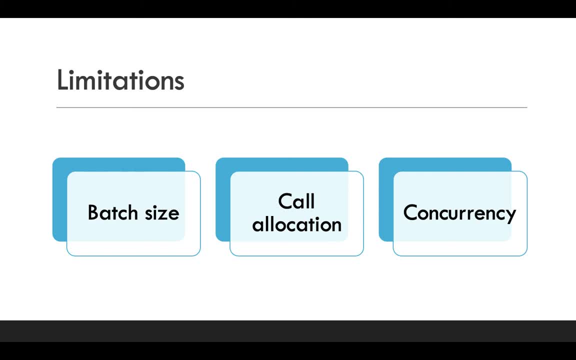 they are doing it illegally, because this is on you, as a human being, to check the licenses. if it is all. if it is possible to scrape the data from a website that the plug-in really doesn't care what the policies are. it is on to you, as the user, to check all these written notes in the websites. 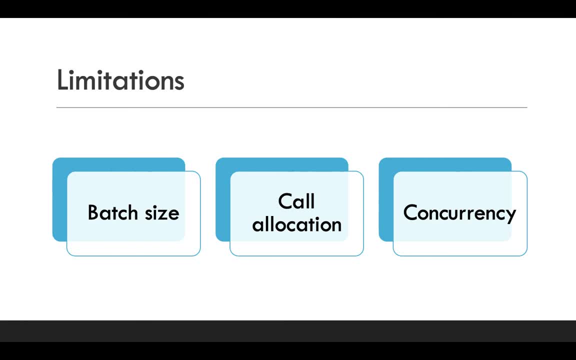 privacy policies that if it is possible to scrape the data. for example, it was some years back- I'm not sure now- but there were plugins that you could use on your Google Chrome and then scraped the information from LinkedIn, but then LinkedIn basically very straightforward said it's in its privacy policy that you really could not scrape the data. so this: